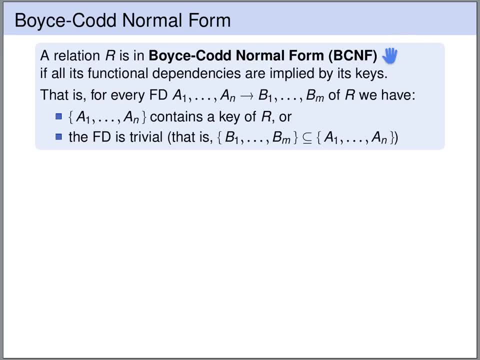 Boyce-Codd- normal form if all of its functional dependencies are implied by its keys. So what does this mean? For every functional dependency of R, one of the following conditions must hold: Either the left-hand side of the functional dependency contains a key of the 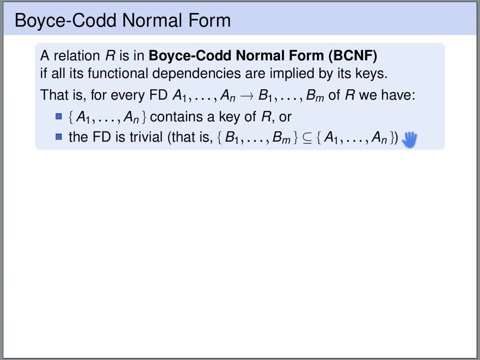 relation R or the functional dependency is trivial and this means that the right-hand side is a subset of the left-hand side. In the first case, if the left-hand side contains a key, the key uniquely determines all of the attributes of the relation. so, in particular, the key uniquely determines the attributes. 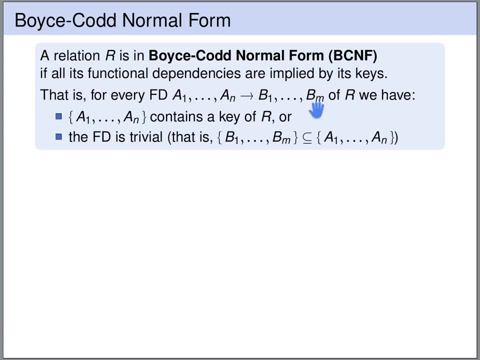 of the right hand side, b1 up to bm. so this key implies the functional dependency. In the second case, our functional dependency is trivial. the right hand side is a subset of the left-hand side and trivial dependencies are always implied by any set of functional. 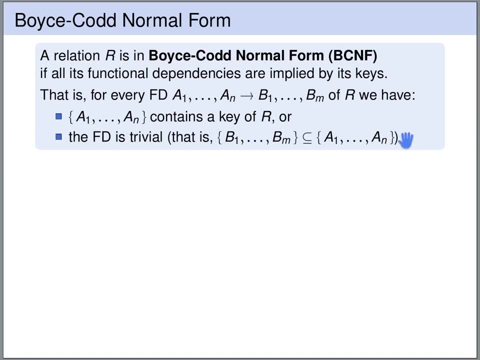 dependencies. So clearly, in both cases this means that the left-hand side, between b1 up to bn and the cases these function dependencies are implied by the keys of the relation R. So this is the two conditions that we have to check. The left-hand side contains a key. 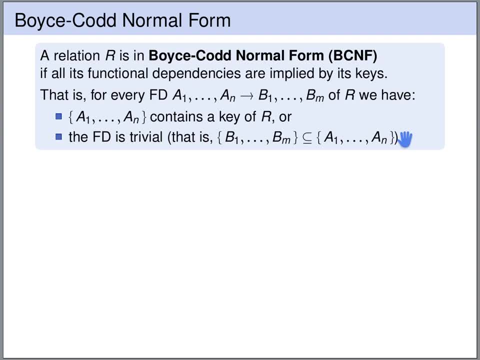 or the function dependency is trivial. Let's have a look at an example Here. we have again our courses table with course number, title, instructor and phone number of the instructor, And we have two function dependencies. The course number uniquely determines the title. 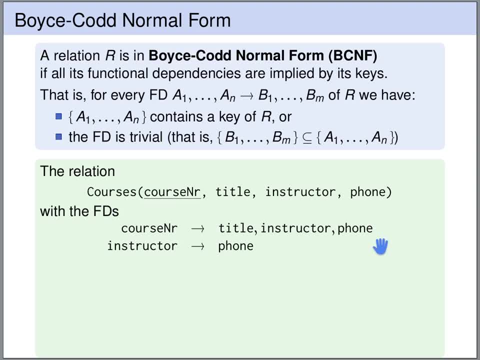 the instructor and the phone And we have a function dependency- that the instructor uniquely determines the phone number. Now is this table in Boyce-Codd normal form. The first function, dependency. the left-hand side contains a key. The course number is a key of this relation. So if we would not 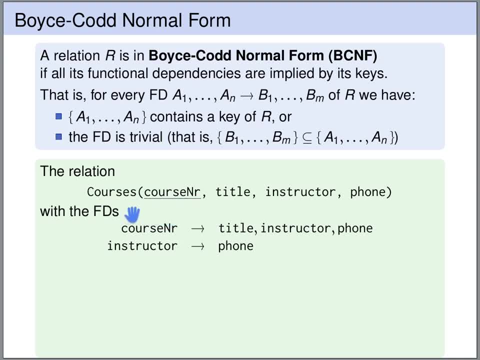 know that the course number is a key. how would we determine this? We would take the left-hand side And we would take the left-hand side And we would take the left-hand side and we would would compute the cover, The cover of the left-hand side, if it contains all the attributes. 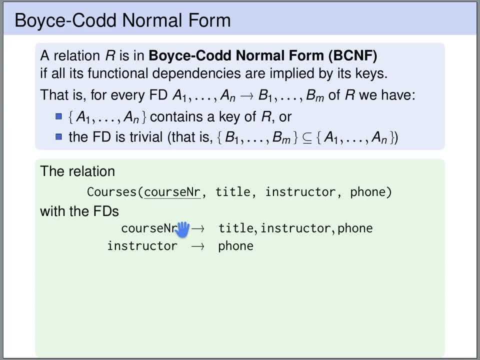 of the relation, then the left-hand side contains a key. If we compute the cover of course number, then we get course number, title, instructor and phone. so we get all the attributes. so indeed, the left-hand side contains a key. So the first function, dependency, is fine. 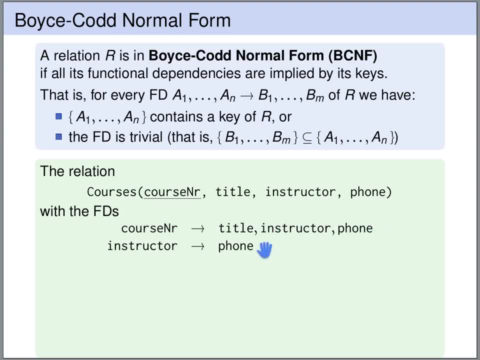 It's implied by a key. The second function, dependency. The left-hand side is instructor. Is this a key of this table? Let's check: If we take the set only containing instructor and we compute the cover, what do we get? We get instructor and phone and nothing else. 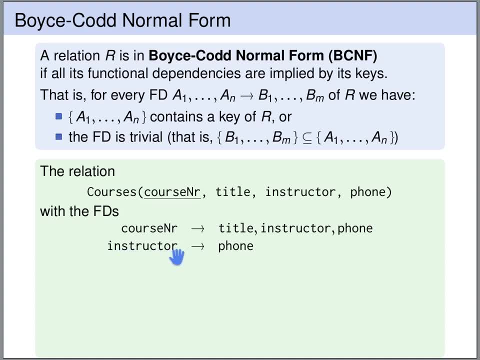 So this is not a key of this table. So we are not in the first case. Let's check whether we are in the second case. Is it a trivial function dependency? The right-hand side is not a subset of the left-hand side, so it's also not a trivial function dependency. So 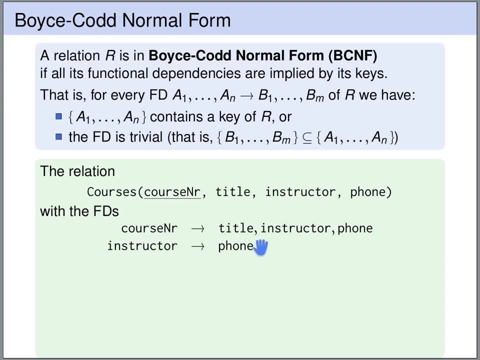 this is not a trivial function dependency. So this is not a trivial function dependency. It is neither implied by a key nor trivial. so it violates the Boyce-Codd normal form. So this table is not in Boyce-Codd normal form. However, if we drop the phone number from, 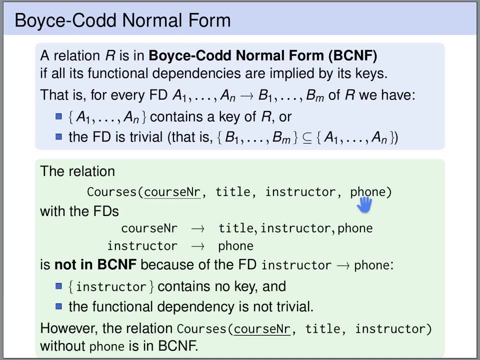 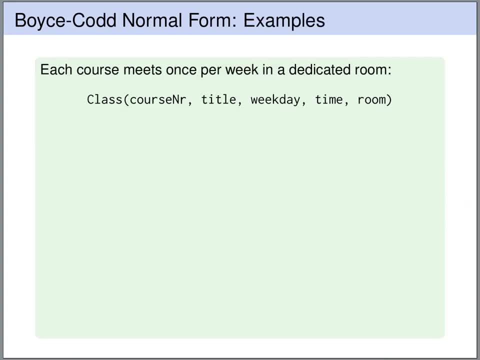 the table. then the resulting table is in Boyce-Codd normal form. Let's have a look at another example Here. we have a table for courses that meet once per week in a dedicated course. So we have a table called class. There is a course number. Every course meets once per 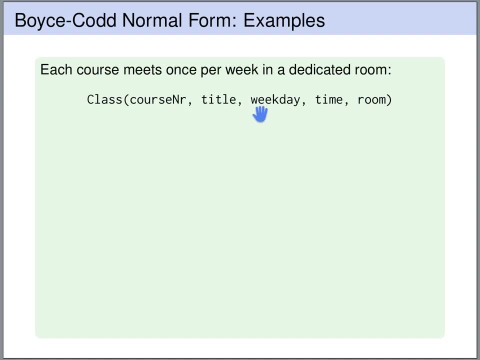 week The course has a title And for the meeting we have a weekday when the meeting happens, a time and the room in which the meeting will happen. So what are the functional dependencies that we would expect to hold If the courses only? 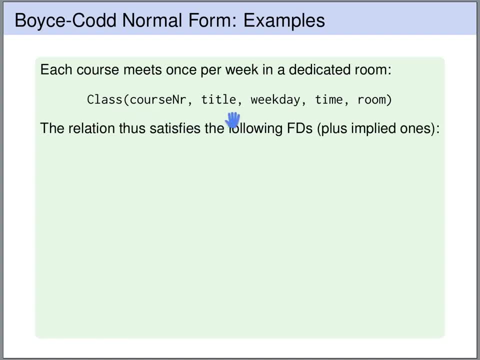 meet once per week, then the course number uniquely determines the weekday, the time and the room. So we have a table called class, There is a course number, Every course meets room. The course number, of course, also uniquely determines the title of the course. Moreover, 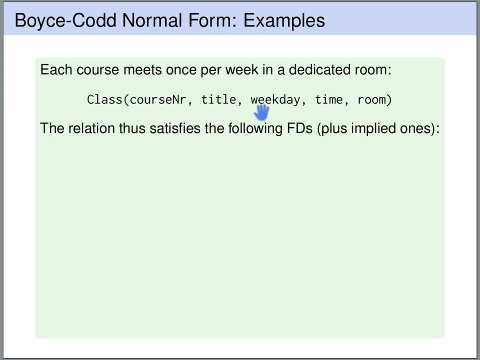 if the course is once per week, then the weekday, the time and the room is enough to know what course we are talking about. So we have two functional dependencies: the course number determines everything, and weekday time and room number determine also everything determine. 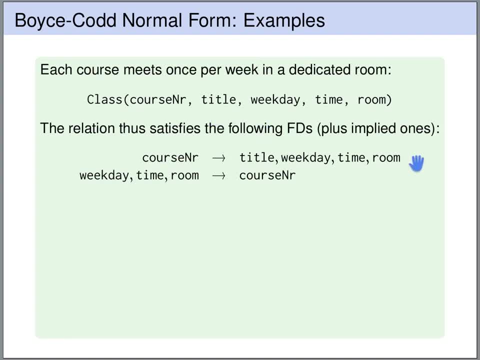 the course number and therefore also the title and so on. So these two functional dependencies imply all other functional dependencies that are valid for this table. Now, what are the minimal keys for this relation? First of all, the course number uniquely determines everything, so the course number on itself is a key. Moreover, the weekday time room. 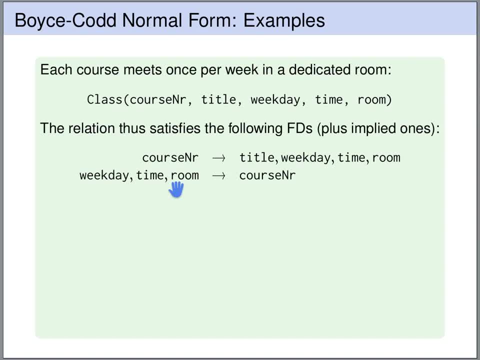 determines the course number. so weekday time room together determines the course number. This is also a minimal key for this relation. We cannot drop anything. we cannot drop the weekday, we cannot drop the time, we cannot drop the room without losing that. 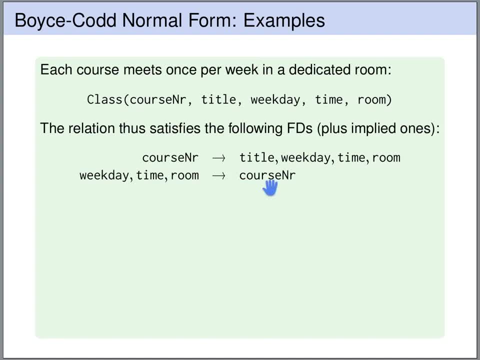 the course number is uniquely determined. So we have two minimal keys, we have course number and we have the weekday time and room. Now it's obvious that if we look at these two functional dependencies, then both of them are implied by keys. 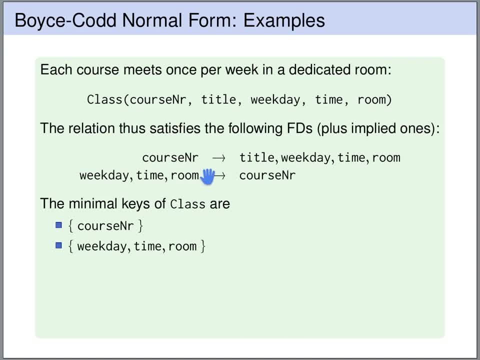 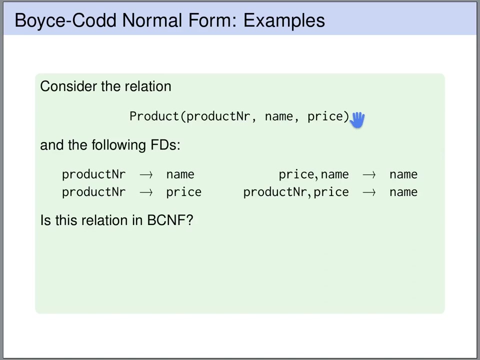 The first one contains this key in the left hand side and the second, functional dependency, contains this key in the left hand side. So both functional dependencies are implied by keys. thus the relation is in Boyce-Codd, number 4.. Let's have a look at one more example. Here we have a table with products, each product. 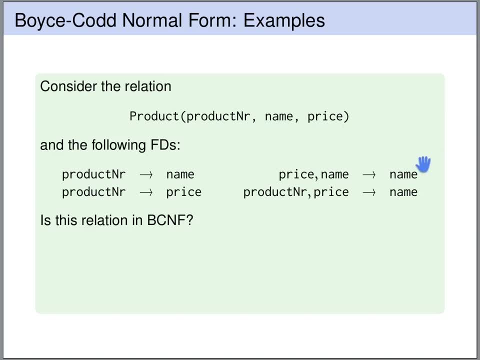 has a product number, a name and a price, And we have these functional dependencies. The product number uniquely determines the name. it also uniquely determines the price. price and name uniquely determine the name, and product number and price uniquely determine the name. Now is this relation in Boyce-Codd normal form? 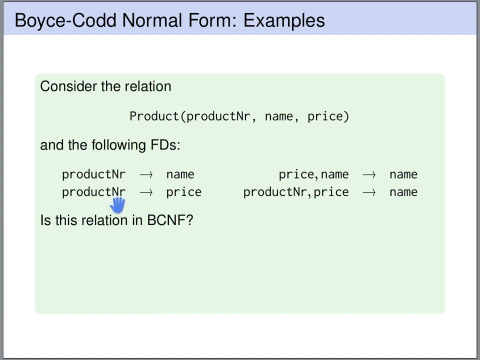 First of all observe that the product number is a key for this relation. The product number uniquely determines the name and price, so it determines all other attributes of the product. So the product number is a key. Now let's have a look at the functional dependencies. 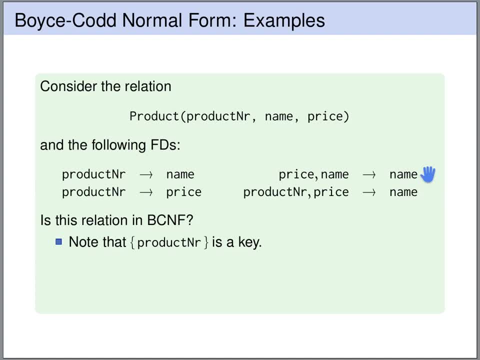 Then we see that we have one trivial functional dependency, namely price name uniquely determines name. The right hand side is a subset of the left hand side, so this one is trivial and we may ignore it. All other functional dependencies- this one, this one and this one- are in the 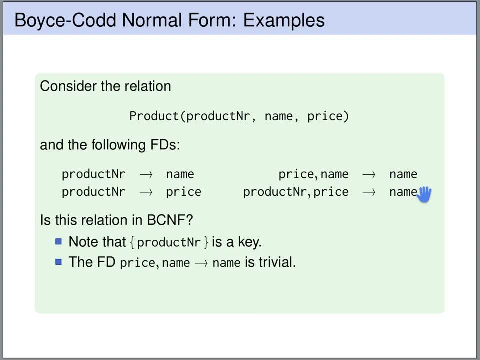 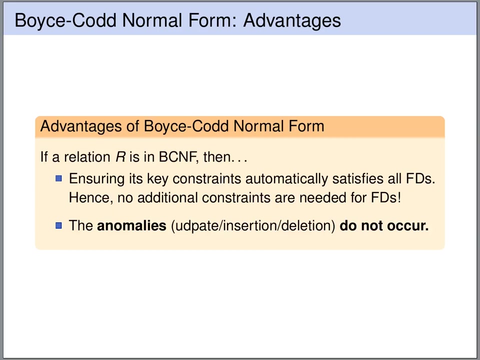 left hand side. So every functional dependency is implied by a key or is trivial. so this relation is in Boyce-Codd normal form. If a relation R is in Boyce-Codd normal form, then enforcing the key constraints automatically satisfies all functional dependencies, So we do not need additional constraints to. 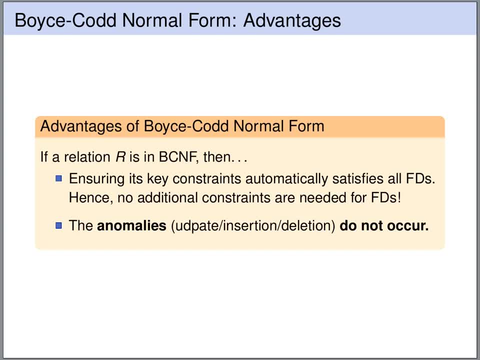 ensure the integrity with respect to the functional dependencies. Also, if a relation is in Boyce-Codd normal form, then the anomalies that we've discussed- the update, the insertion and the deletion anomalies- do not occur. Let's have a look at two more examples. 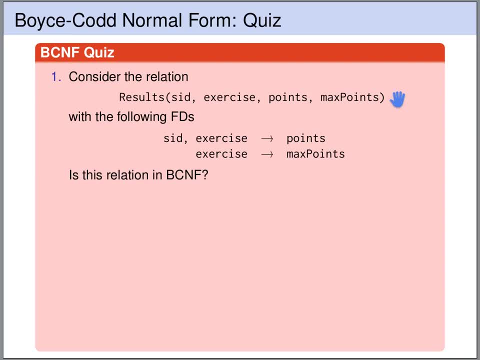 Here we have a relation. results with attributes: sit- the student ID. exercise, the exercise number points- the number of points the student has obtained on the exercise. and max points, the maximum number of points available for the exercise. For this relation, we have the following functional dependencies: Sit and exercise together uniquely. 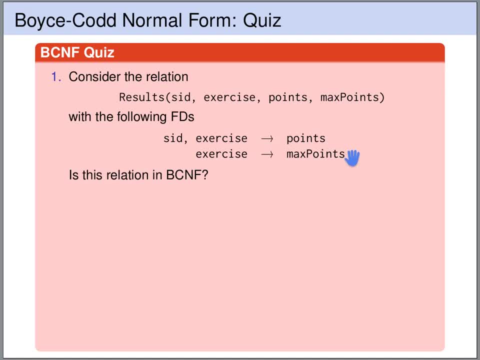 determine the points and exercise uniquely determines the max points. These two functional dependencies together imply only that the function is in Boyce-Codd normal form, So apply all other functional dependencies. Now is this relation in voice code normal form? Let's have a look at the first functional dependency, the left-hand side. sit and exercise. 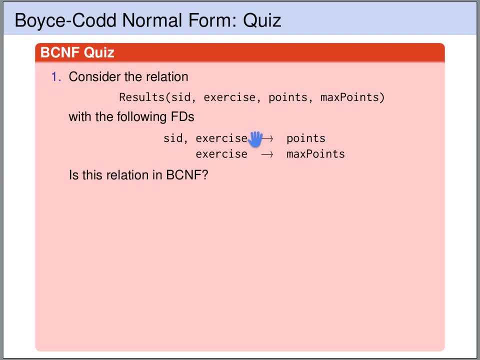 Does it contain a key? In order to check this, we simply compute the cover of the left-hand side. So we take sit and exercise and we compute the cover, We get the points and from the exercise we get the max points. So indeed, the cover contains all the attributes of the relation. so the left-hand side contains: 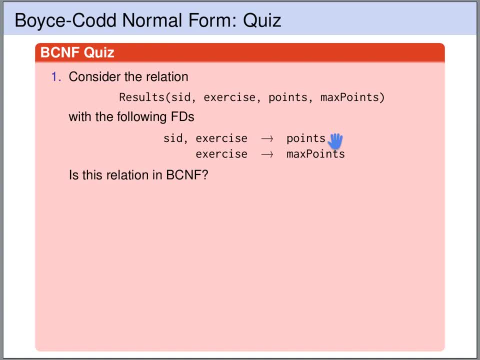 a key. So the first functional dependency is fine. Now let's have a look at the second functional dependency. The left-hand side is exercise. If we compute the cover of exercise, we only get exercise and max points, nothing else. So the left-hand side is not a key. 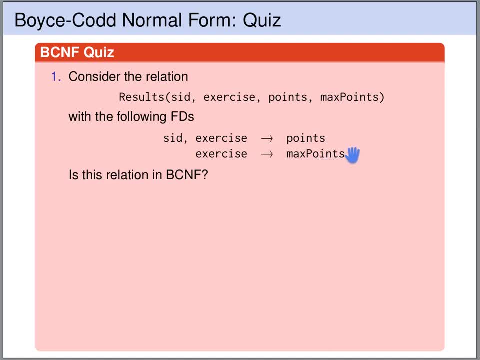 It does not contain a key. Also, this functional dependency is not trivial. The right-hand side is not a side. The left-hand side is a subset of the left-hand side. So this functional dependency violates the voice code normal form. It's not implied by a key. 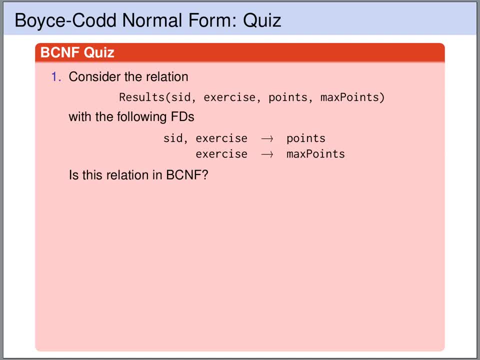 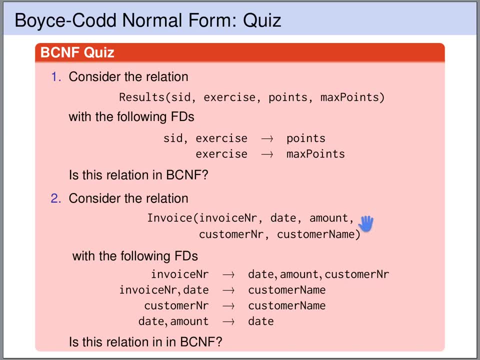 So this relation is not in voice code normal form. The second example is a table with invoice information. We have an invoice number, a date of the invoice, the amount of the invoice, the customer number and the customer name And we have the following functional dependency: 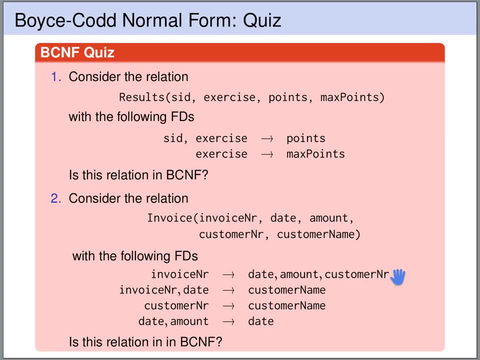 The invoice number uniquely determines the date, the amount and the customer number. So let's have a look whether this functional dependency is in voice code normal form. We have a look at the left-hand side, the invoice number. Let's check whether the invoice number contains a key of this relation. 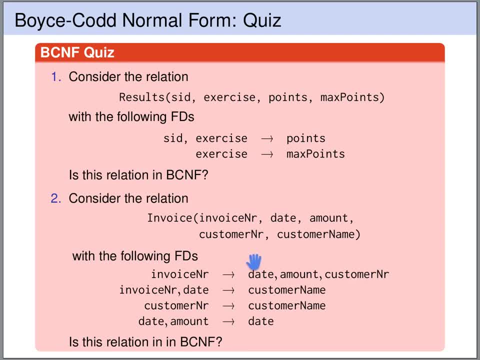 So we compute the cover of invoice number, We get the date, the amount and the customer number, And because of the customer number, we also get the customer name in the cover. So indeed, the cover of the left-hand side contains all the attributes of this relation. 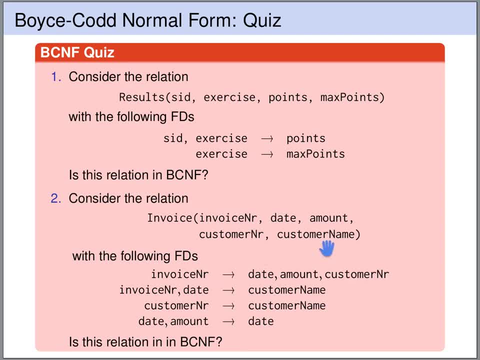 So the invoice number is a key of this relation. So the first functional dependency is fine. Likewise, the second functional dependency contains the invoice number on the left-hand side, so it also contains a key of this relation. So this functional dependency is fine as well. 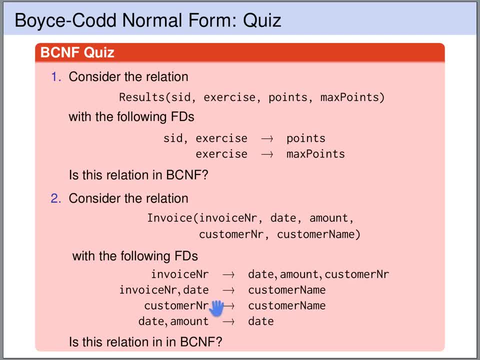 Let's have a look at the third functional dependency. Here we have the left-hand side, the customer number. Let's compute the cover of the customer number and we get the customer name and nothing else. These two functional dependencies are not applicable and also this one is not applicable. 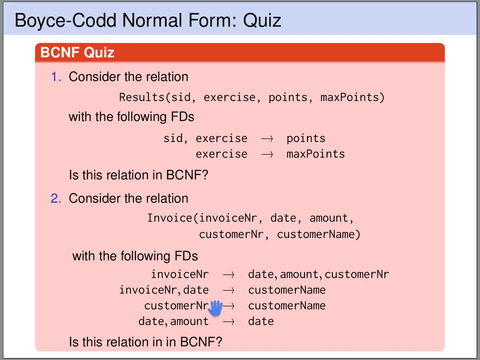 So the cover of the customer number only gives us customer number and customer name, so this is not a key of this relation. Is this functional dependency trivial? No, the right-hand side is not a subset of the left-hand side, So it's non-trivial and it's not implied by a key. so this functional dependency violates.